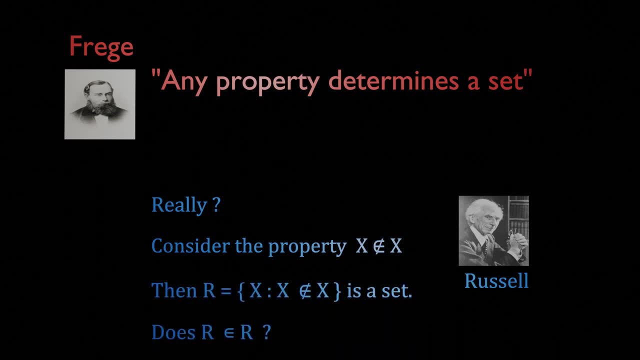 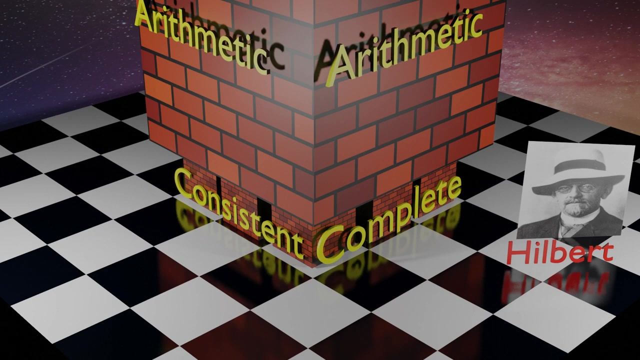 a way to find a solution to the problems of mathematics, including explicit counter-examples. Consider, for example, the paradoxes and contradictions in the early set theory. Many found a lot of these developments deeply troubling. A foundational crisis arose. Hilbert, one of the leading mathematicians of the late 19th century, proposed a way to find a 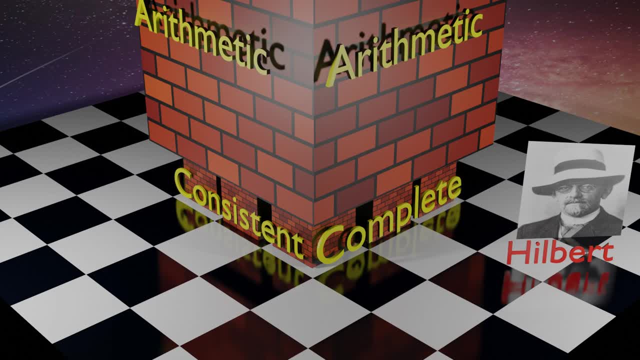 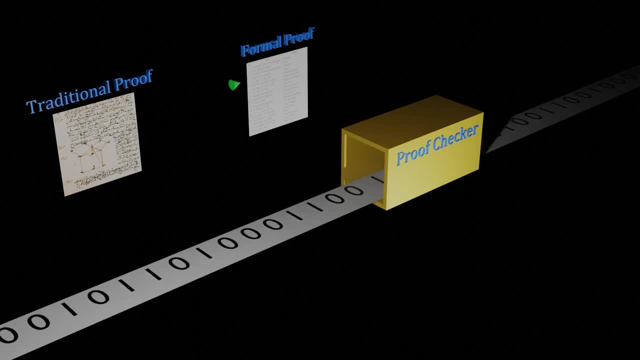 solution. Hilbert proposed to find a consistent and complete proof that it was both complete and consistent. In order to be able to accomplish this, however, one needed to have some way to study proofs and mathematics itself. There arose the notion of formal proof. 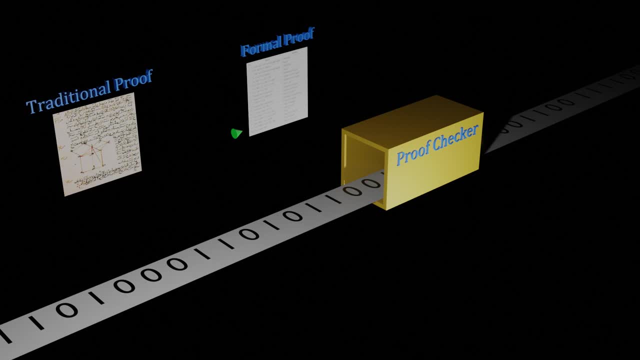 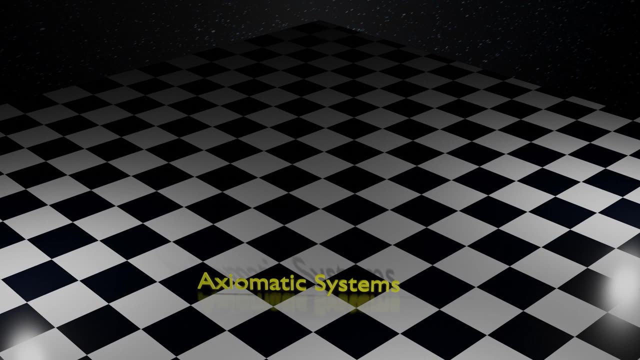 the idea of an axiomatization of basic mathematics. There were several competing axiomatic systems for the basics of mathematics. Zermelo attempted to axiomatize set theory, later expanded to Zermelo-Fraenkel set theory. Gettler's axiomatic allowing learn success. 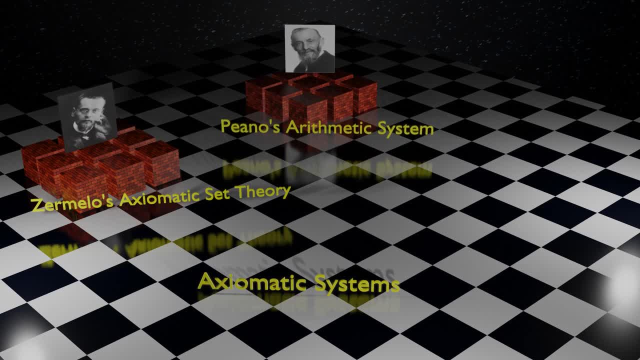 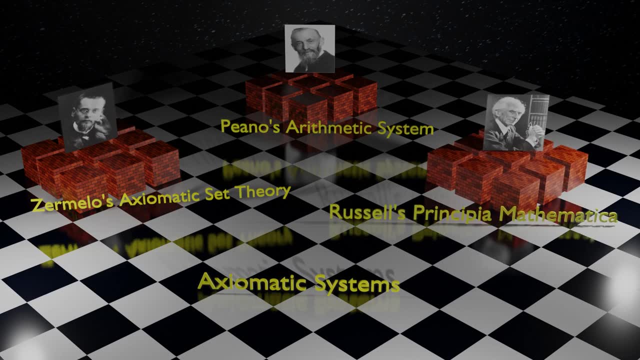 Peano had proposed a collection of axioms for basic arithmetic and, famously, Russell and Whitehead had, in their massive book Principia Mathematica, attempted to establish an axiomatic and deductive system for all of mathematics. Some early successes were achieved, with people showing that some parts of such theories were 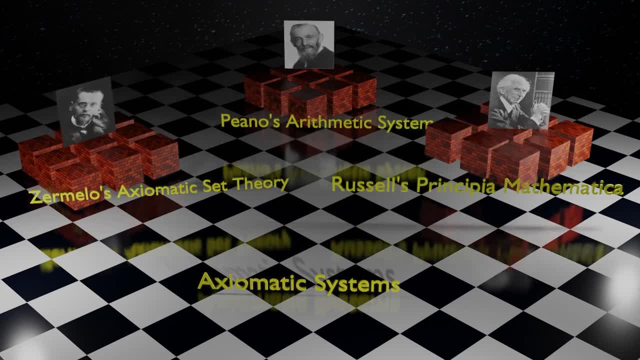 in fact consistent. The stations were made for certain points with 17, ilebrush was challenging and thepurė largeanı. Then came Getull's result. A hectic rehearsal was carried out in an attempt to get to get too much flow, relatively room by the krieg to launch the ambush. 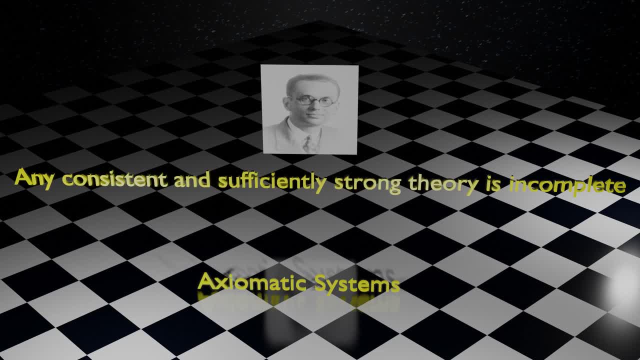 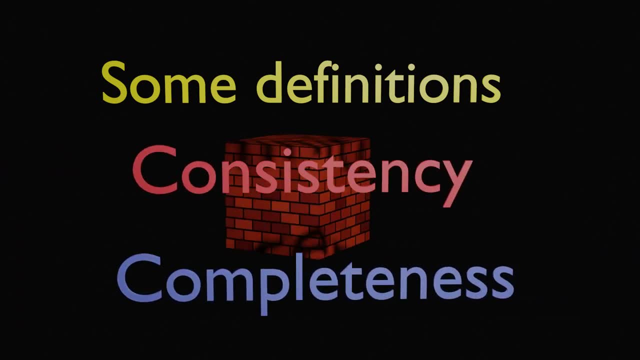 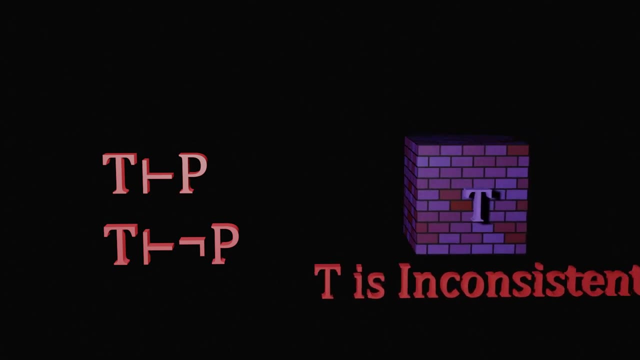 consistent and sufficiently strong theory is incomplete. But let's start with some definitions. What are consistency and completeness? We say a formal theory is consistent if you cannot prove both a sentence and its negation. In fact, because from P and no P you can prove anything using classical logic. it is equivalent. 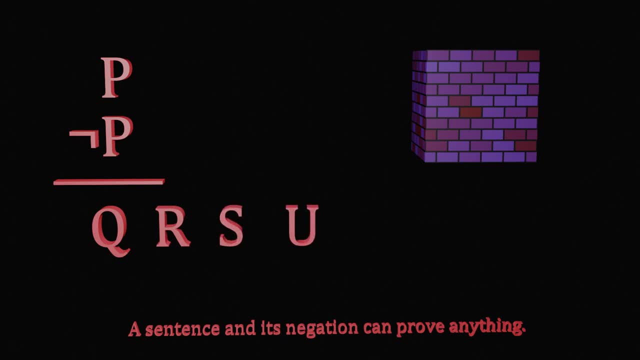 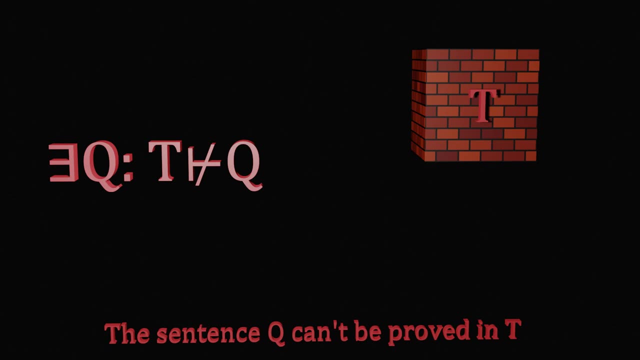 that a theory is consistent if, and only if, there is at least one sentence queue, such that there is no proof of queue in the theory. By contrast, a theory is said to be complete if, given any sentence P either, there is a. 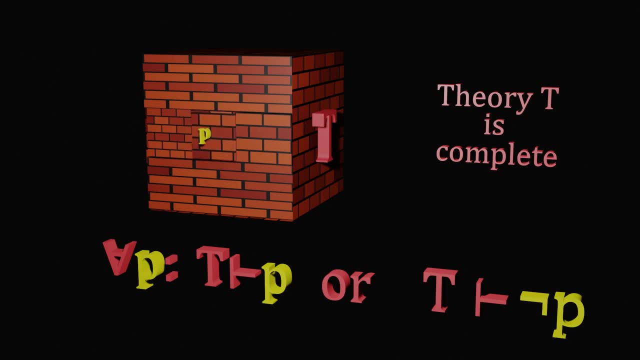 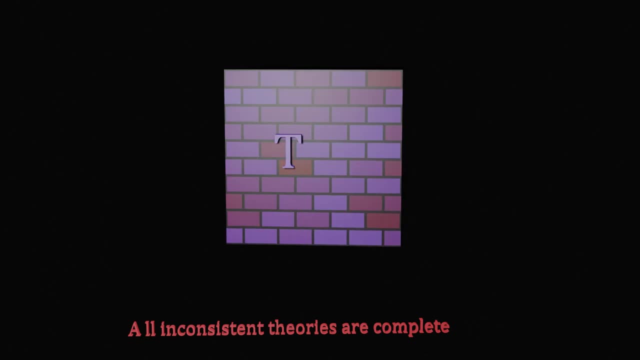 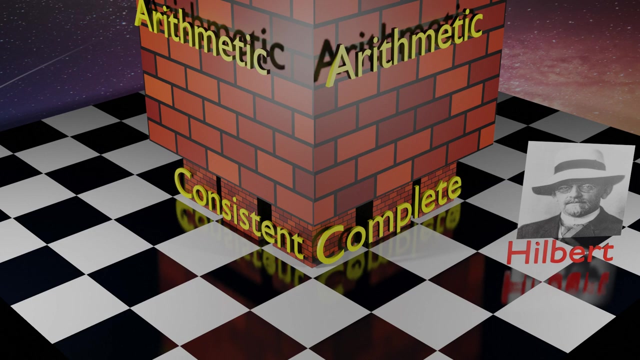 proof of P or a proof of no P. Note that an inconsistent theory is necessarily complete. Remember that Hilbert proposed to find a consistent and complete axiomatization of arithmetic, together with a proof that it was both complete and consistent. So let's see what an axiomatic system is. 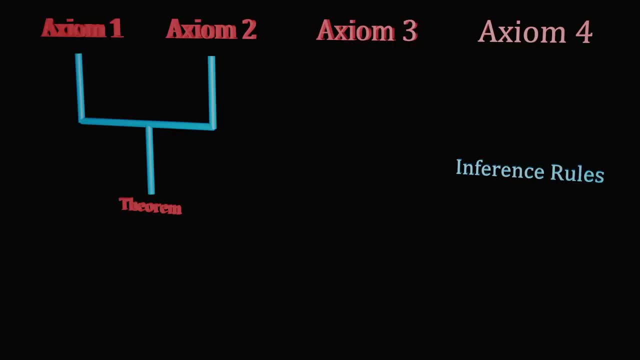 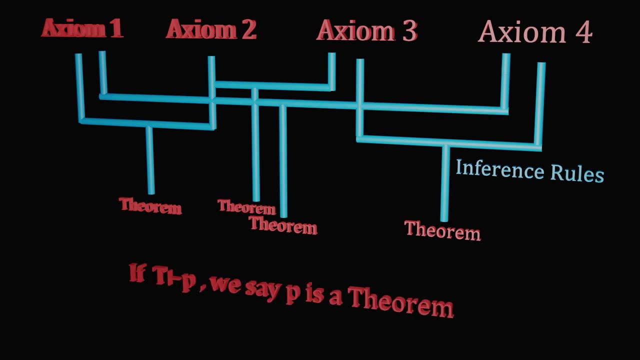 An axiomatic system is any set of axioms from which can be used to derive theorems according to a set of rules. We will say that a sentence is a theorem of the theory if there's a proof of the sentence from the axioms of the theory using the inference rules. 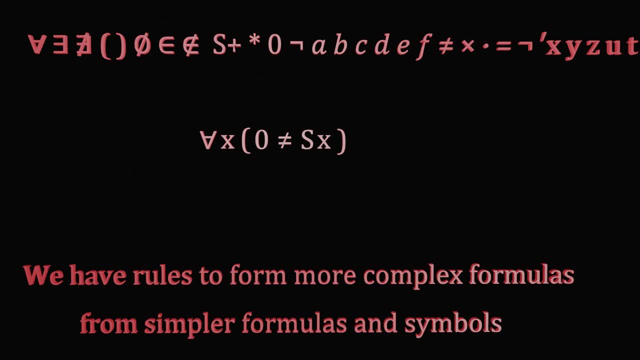 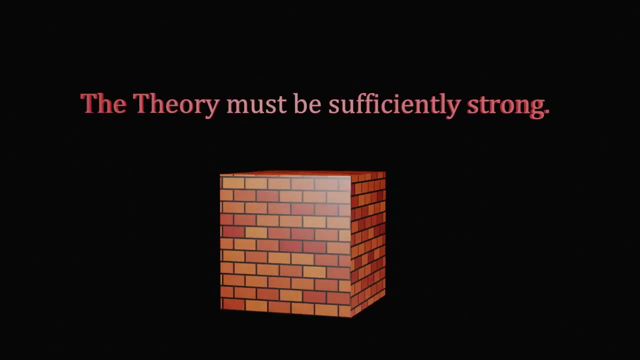 Each formal system is described by primitive symbols which collectively form an alphabet and which can be used to construct a formal language. Then we can build valid formulas through finite combinations of the primitive symbols. Gödel's theorem also demands that the theory is sufficiently strong. 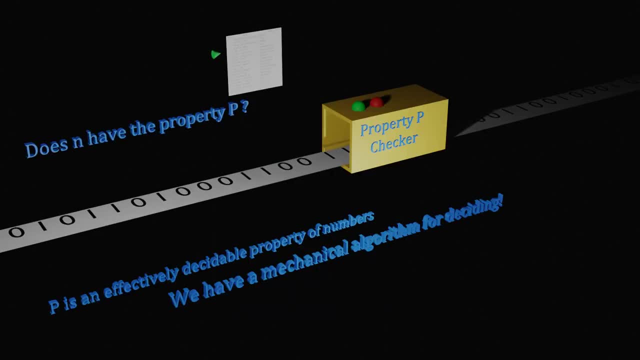 What does that mean? Suppose that P is some effectively decidable property of numbers, that is, one for which we have a mechanical algorithm for deciding, given a natural number, n, whether n has property P or not. We will mainly want to aim for a formal theory T which has at least the two following characteristics: 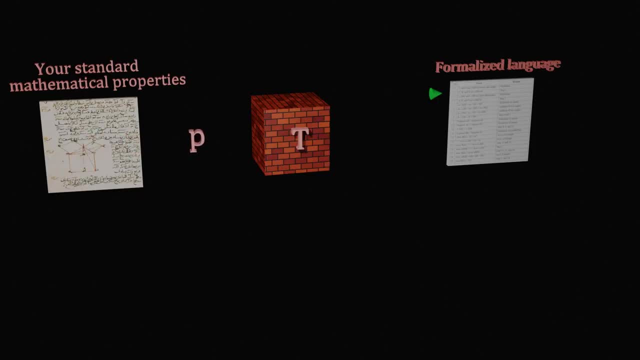 First, the theory T is able to frame some formula Φ which expresses the decidable property P, And second, T is such that if n has the property P, T proves Φ, and if n does not have the property P, T proves no Φ. 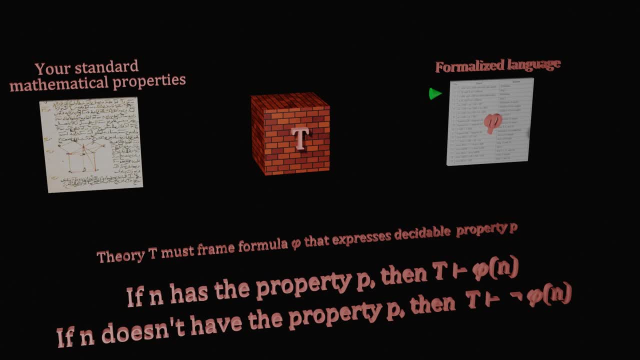 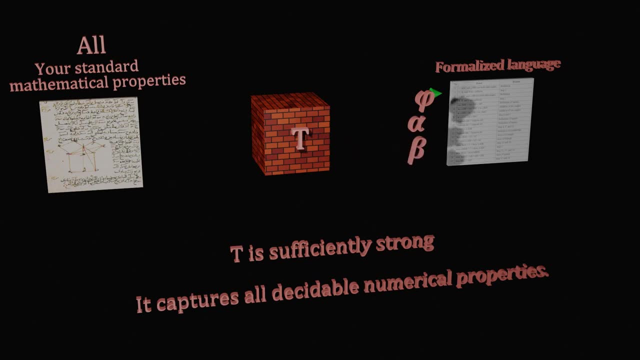 That is, we have the formula P-P-Pi-Pi-Pi. We can say that the formula T is the formula P-Pi-Pi-Pi-Pi. That is, we want t to capture p. Then we say a formal theory of arithmetic: t is sufficiently strong if it captures all. 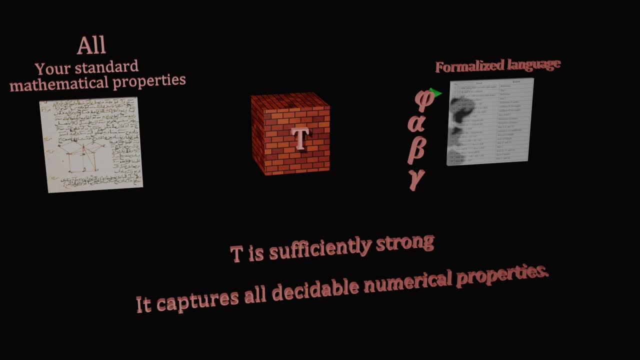 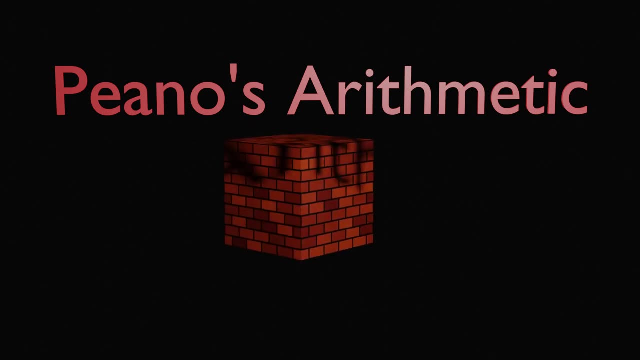 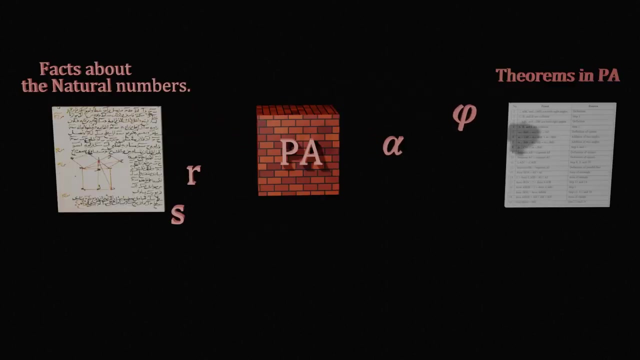 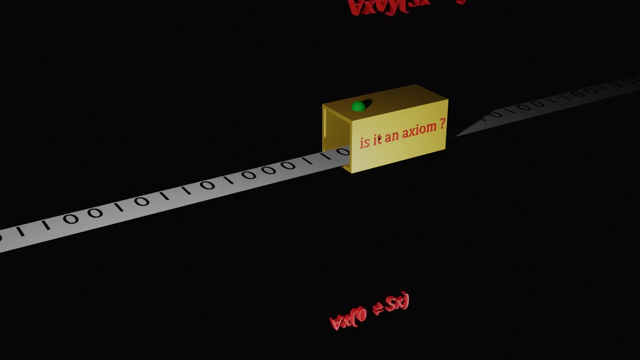 decidable numerical properties. Let's focus our attention to a particular theory, the first-order Peano arithmetic, or PA for short. Peano arithmetic is a rich theory to prove many facts of the natural numbers. It is decidable whether any given formula has the right shape to be one of the axioms. 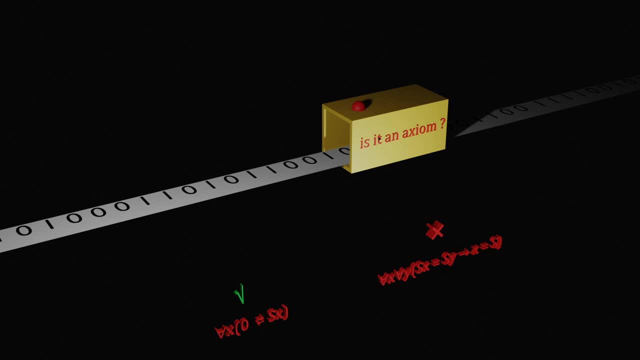 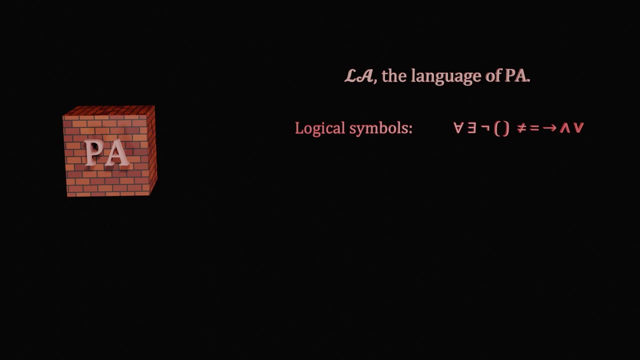 so PA is a legitimate formalized theory. The language of PA is LA, a first-order language. Its non-logical vocabulary comprises just the constant zero, the one-place function symbol s and the two-place function symbol s. 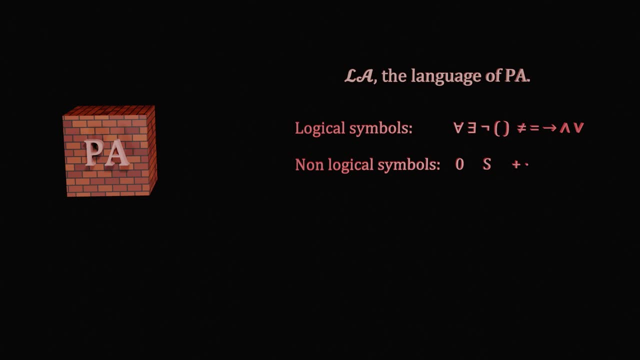 The function symbols plus and times Characters to express variables. The given interpretation is the obvious one. PA's deductive proof system is some standard version of classical first-order logic with identity. Differences between versions aren't significant, For example universal instantiation. 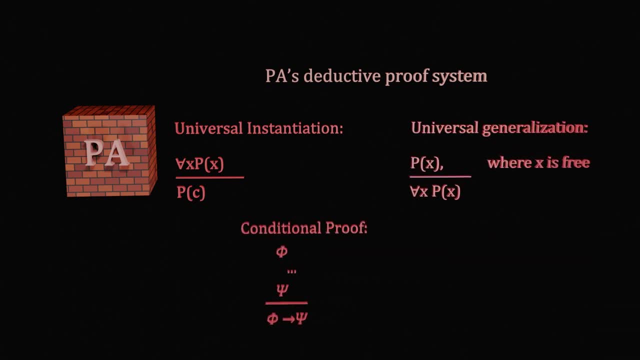 universal generalization and conditional proof. PA axioms are the following sentences: The first axiom says zero is not the successor of a number. The second axiom says s is a one-to-one function. Axioms 3 and 4 define addition. 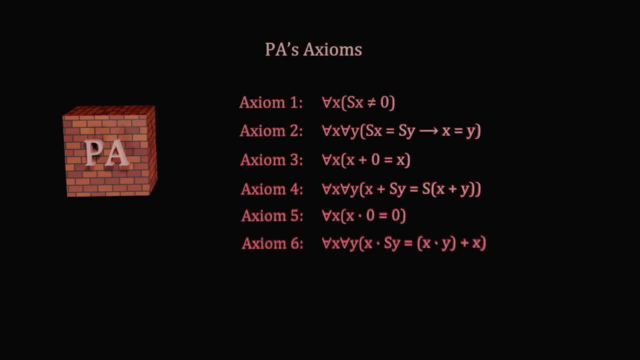 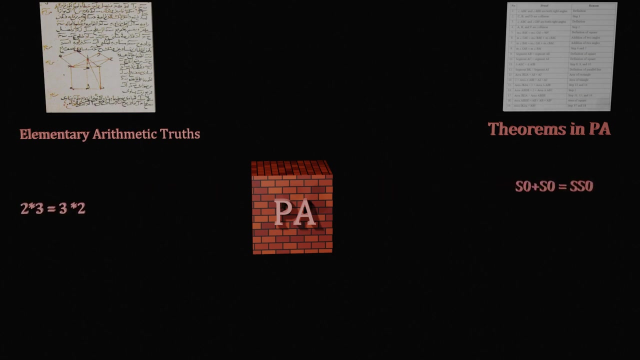 Axioms 5 and 6 define multiplication Plus every sentence, that is, the universal closure of an instance of the induction schema. PA does indeed have the resources to establish all the familiar elementary general truths about the addition and multiplication of numbers. PA has the successor function- addition and multiplication- built in. 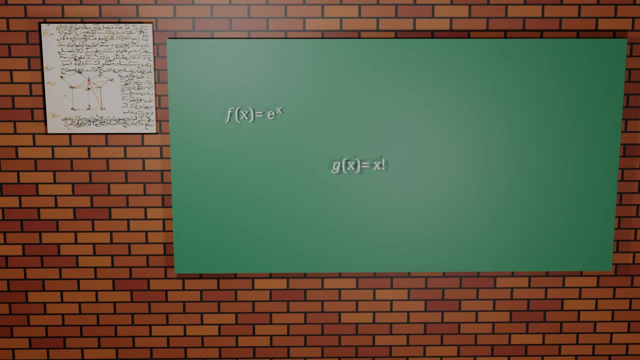 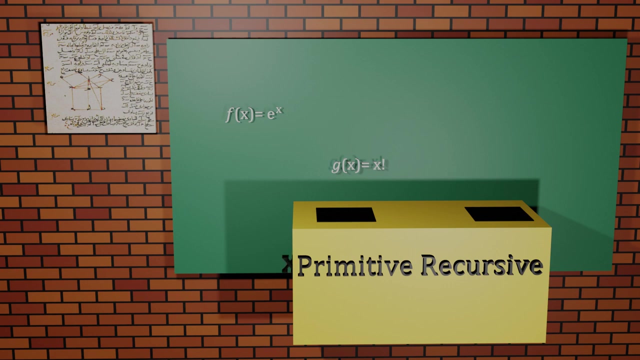 But why on earth stop there? School arithmetic acknowledges many more numerical functions, like exponential, factorial and others. These can be defined or constructed with a special class of functions, the so-called primitive recursive ones, And we'll see that PA in fact already have the resources to deal with all these primitive. 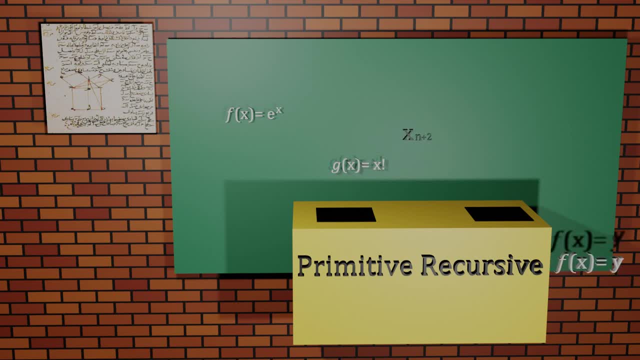 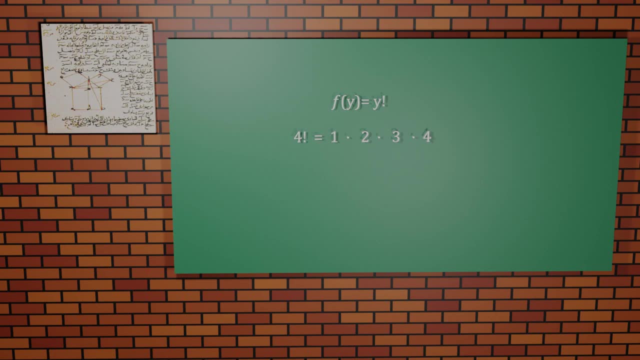 recursive functions. Take the function y factorial where, for example, 4 factorial equals 1 times 2 times 3 times 4.. This can be defined by the following two equations: y factorial equals 1 times 2 times 3 times 4.. 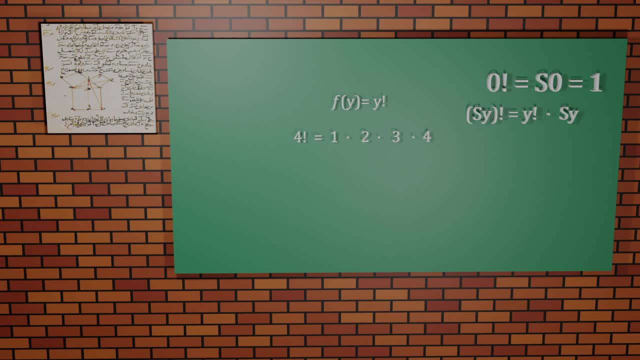 So we're doing this per using the frightened linearization function, just like the regular rhymes and alphabets. The first clause tells us the value of the function, for the argument y equals 0.. The second clause tells us how to work out the value of the function for sy once we 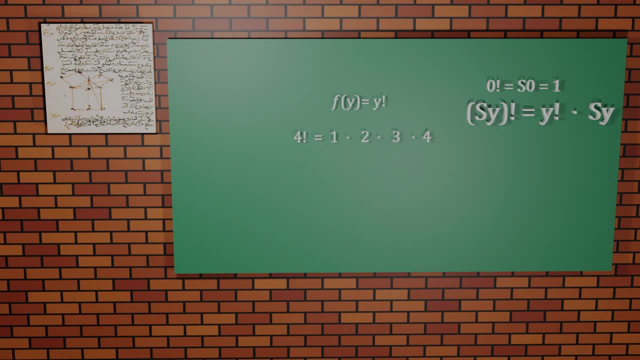 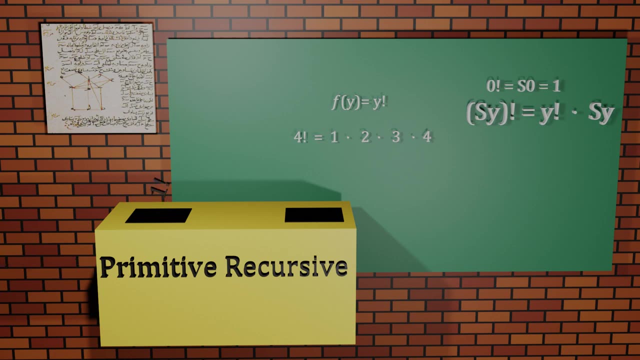 know its value for y and assuming we already know about multiplication. So by applying and reapplying the second clause, we can successively calculate 1 factorial, 2 factorial, 3 factorial, etc. So how do we do that? 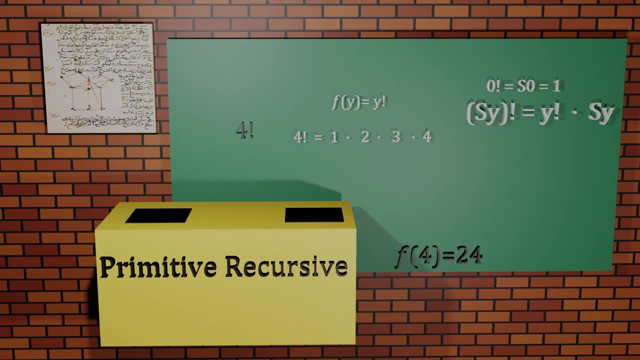 We're going to use an addition whoseounge equals d, So this can be applied. So if D is still an integral value, then the solutions for u are Na and K. A primitive recursive function is one that can be characterized by a chain of definitions, by recursion and composition. 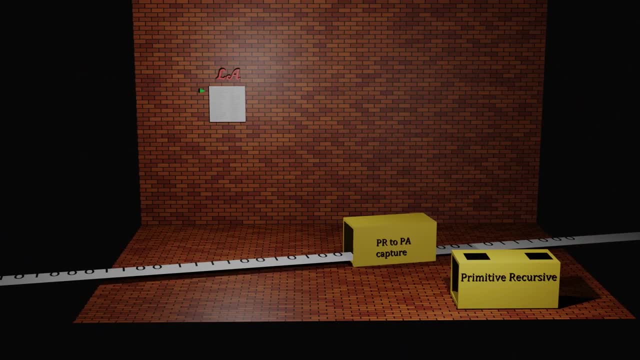 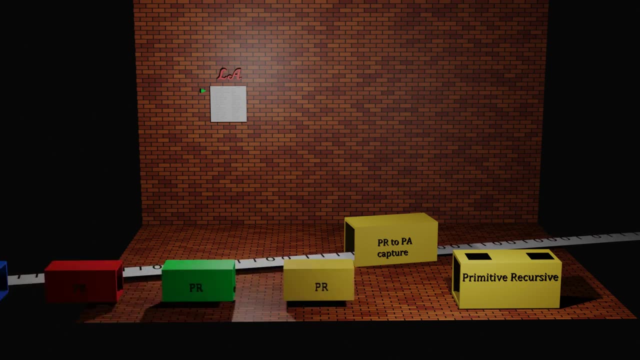 The primitive recursive functions are computable. The composition of two computable functions, f and g, is computable. So as we build up longer and longer chains of definitions for primitive recursive functions, we always stay within the class of computable functions. 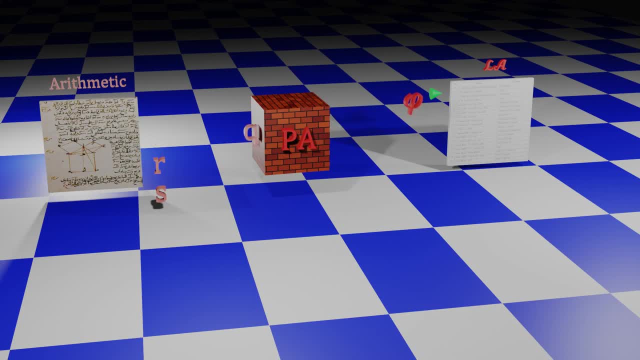 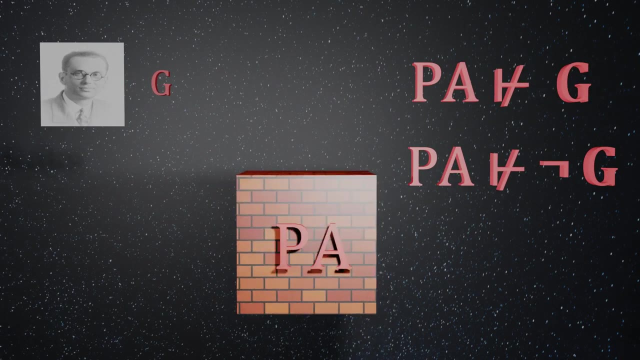 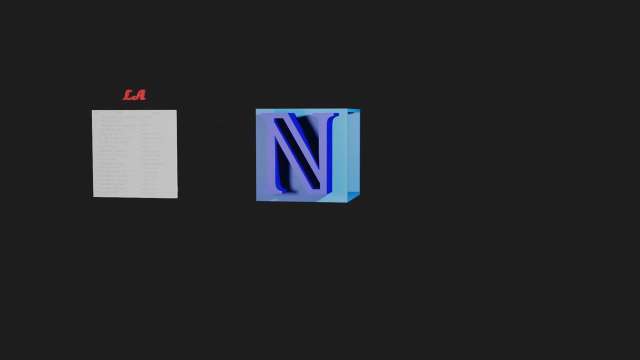 PA can capture all primitive recursive functions. Now that we have an adequate theory capable to formally capture all important functions, we will see how Geddes constructs a sentence that itself, or its negation, can't be proved. First, Geddes will convert the language of the theory into arithmetic, what is called the arithmetization of syntax. 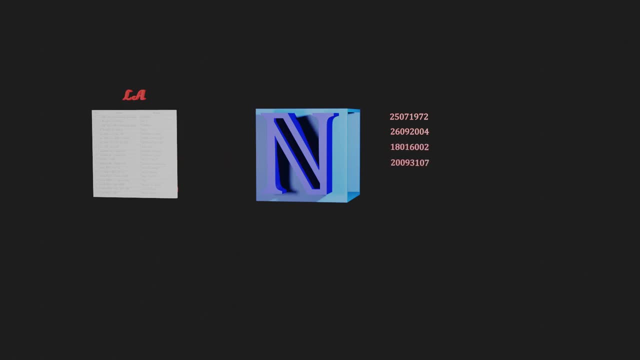 Geddel has the simple but wonderfully powerful idea of associating numbers with the formulas and proofs. from a formal theory We can define the numerical property WFF where it holds, when n is code number in our scheme for a well-formed formula of PA. 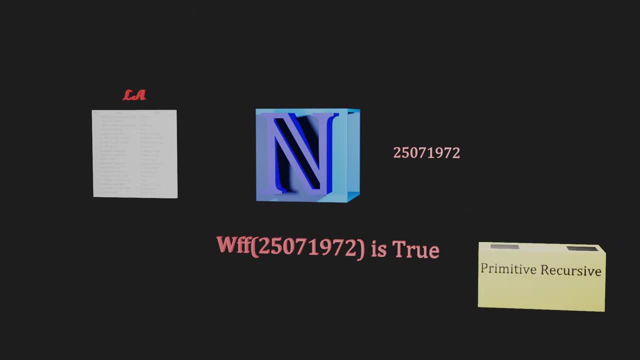 And it will be easy to see that WFF will be primitive recursive. More excitingly, we can define another numerical relation which helps us to compute the formula as a method of GitHub data sisters in our scheme for a well-formed formula of PA. 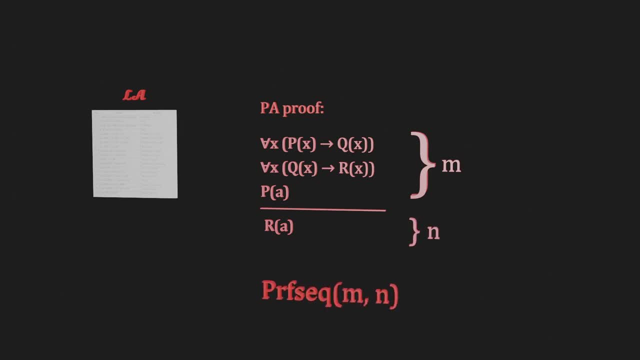 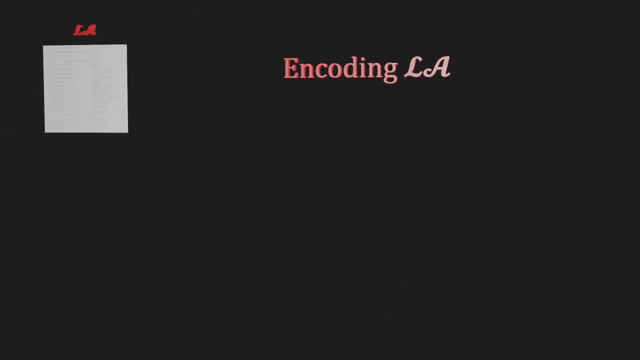 And it will be easy to see that WFF will be primitive recursive. just when m is the number in our scheme of APA. proof of the sentence with number n, We'll start by thinking about how to encode expressions of LA. Suppose that our version of LA has the usual logical symbolism. 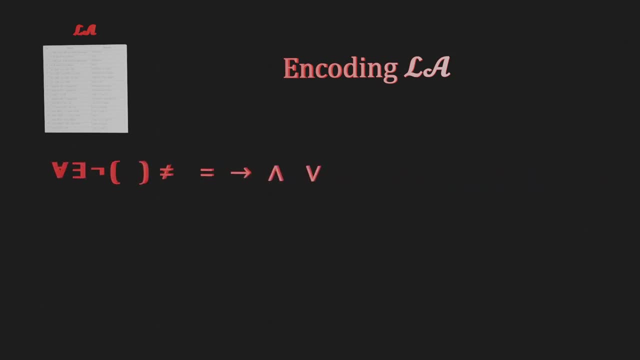 connectives, quantifier symbols, identity brackets and symbols for zero and the successor addition and multiplication functions Associate all those with odd numbers, different symbol, different number. LA also has an inexhaustible supply of variables which we'll associate with even numbers. 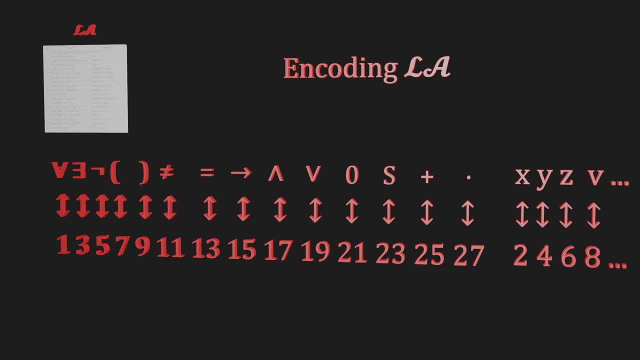 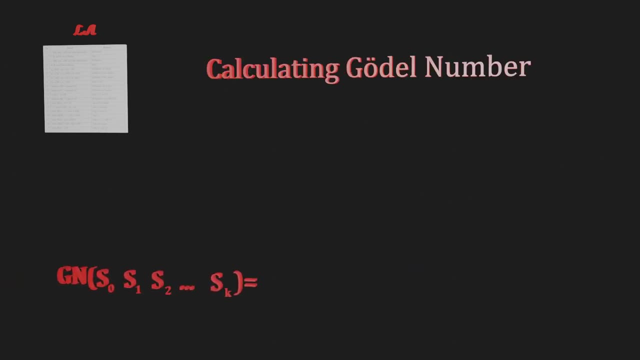 So to pin that down, let's see how we calculate the Gödel number of a formula. Let's say we have a sequence of k plus 1 symbols s0 to sk, Then its Gödel number. The Gödel number is calculated by taking the symbols' correlated code numbers. 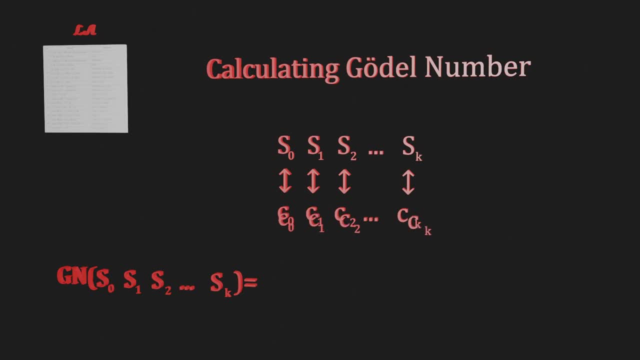 and using them in turn as exponents for the first k plus 1 prime numbers, p0 to pk, and then multiplying the results. Let's see an example. Let's take this sentence from our LA language. The sentence is composed of 12 symbols. 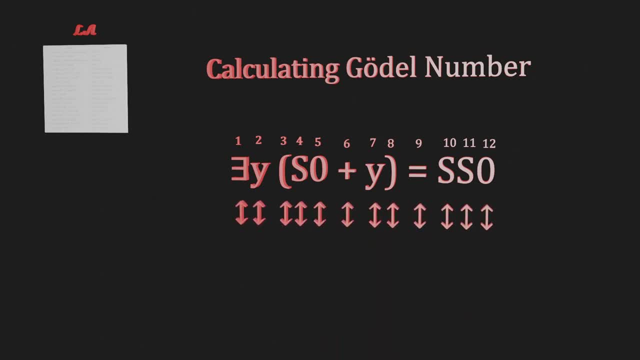 We find the code number for these symbols, We use these code numbers as exponents for the first 12 prime numbers And finally we multiply the result. But now how do we code for proofs? Proofs are simply sequences of formulas. 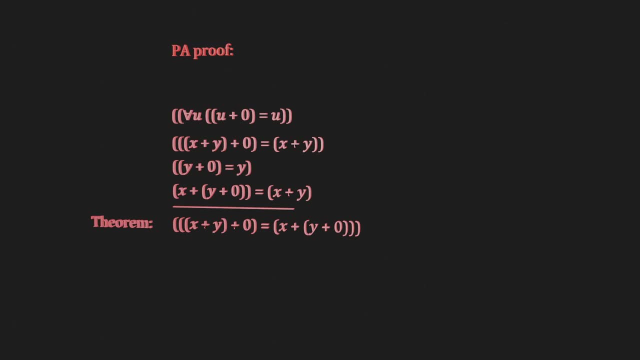 Then a nice way of coding these is by what we'll call super Gödel numbers. So, given a sequence of PA formulas, we first code each to get a regular Gödel number and obtain a resulting sequence of regular Gödel numbers. 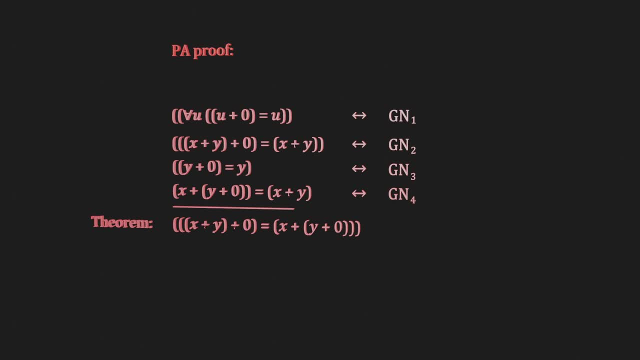 We then encode this sequence of regular Gödel numbers into a super Gödel number. by repeating the trick of taking powers of primes, We can now define more carefully the relation proof sequence which is going to concern us so much. The relation holds just if M is the super Gödel number of a sequence of formulas. 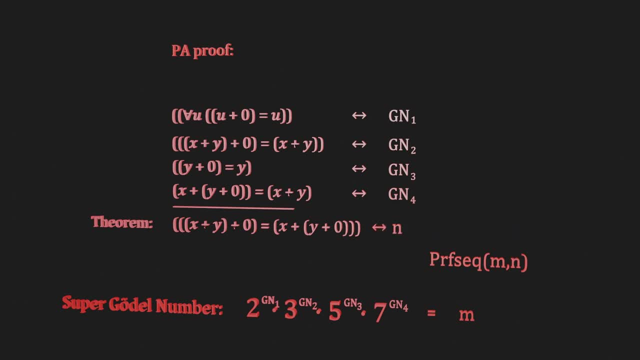 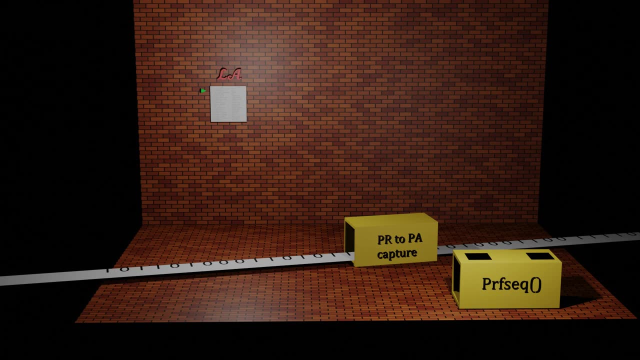 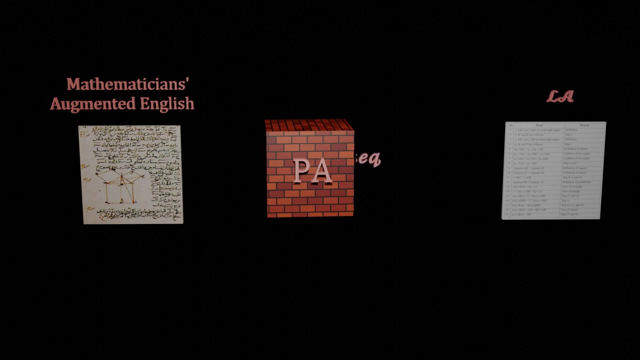 that is a PA proof of a closed formula with regular Gödel number n. The relation proof sequence is primitive, recursive and therefore can be captured by the language of the theory. So in capturing these kind of functions one can talk about the theory from within the theory, using its own language. 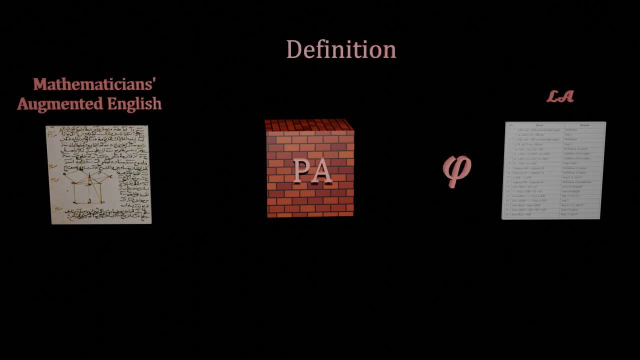 Let's introduce some useful notation. If phi is an LA expression, then we'll use phi in between square brackets to denote phi's Gödel number. Borrowing a species of quotation mark is appropriate, because this number can be thought of as referring to the expression phi in our coding scheme. 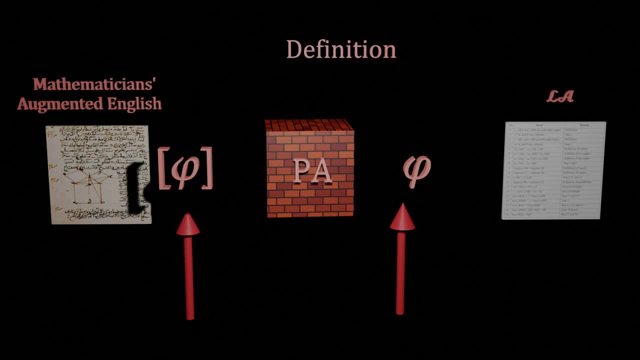 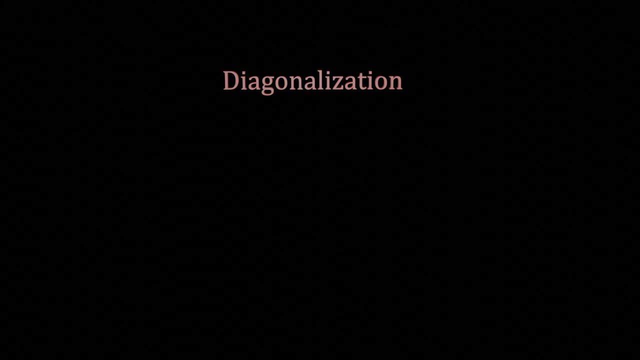 An important step to construct the desired Gödel sentence is called diagonalization. Gödel's construction involves taking a particular open formula that we'll abbreviate u or by u- y when we want to emphasize that the variable y is free. this is not bound by a quantifier. 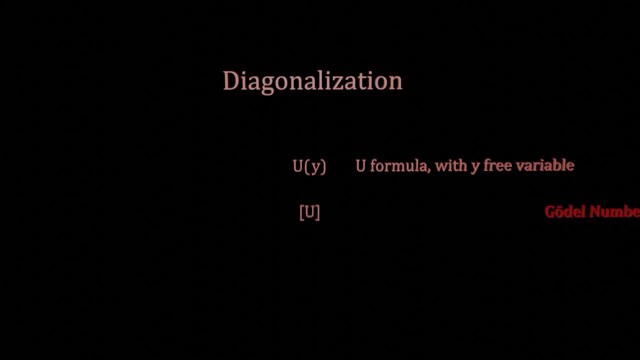 This formula has this Gödel number, Then Gödel substitutes this numeral for the free variable in u. So the key step involves forming this formula. We have taken the free y variable from the original formula and replaced it for the Gödel number of the formula. 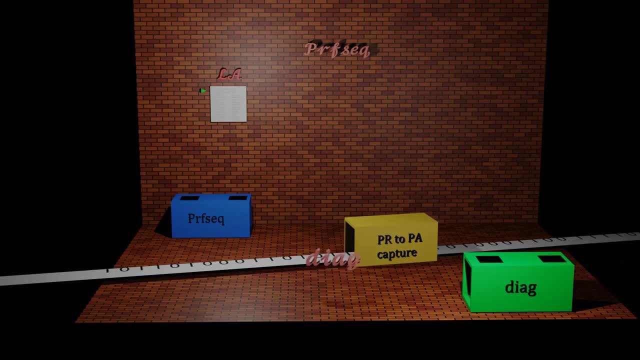 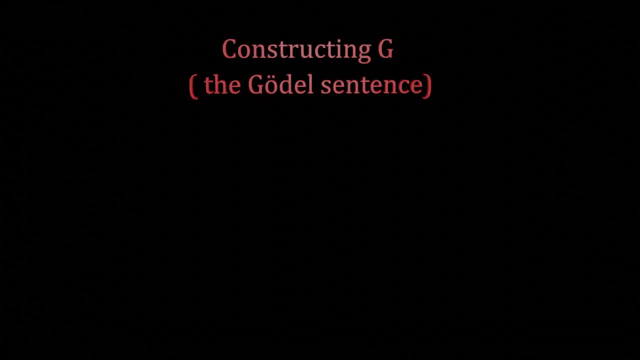 The diagonalization function is also primitive, recursive, so it can also be captured by the language of the theory. Now consider the following relation, which will play a starring role in the Gödel's sentence construction. We define the GDL relation as the composition of the two relations: proof, sequence and diagonalization. 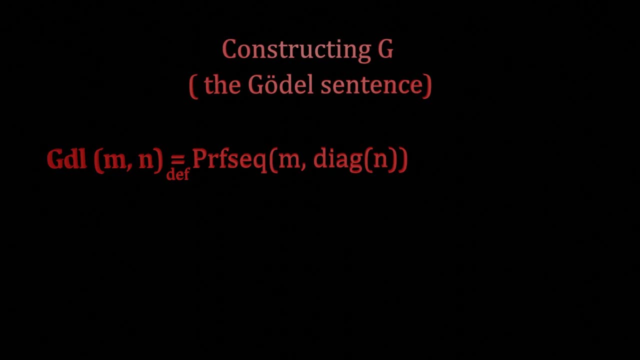 When does this relation hold? Evidently, it holds when m is the super Gödel number for a proof of the diagonalization of the formula with Gödel number n. Given that proof, sequence and diagonalization are indeed primitive recursive, GDL is primitive recursive by composition of functions. 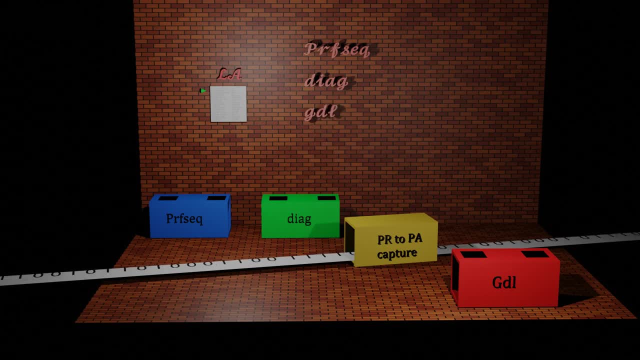 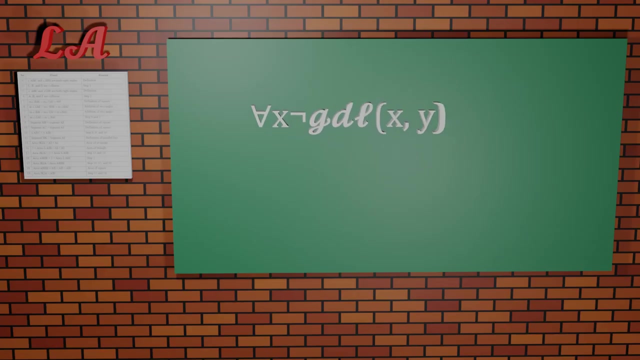 The pieces we need are at long last all in place, So we can finally give Gödel's quite beautiful construction, which delivers a true but unprovable sentence for PA. Consider then this PA formula, Abbreviate this formula as UY, and remember- we want to stress- that it contains just Y, free. 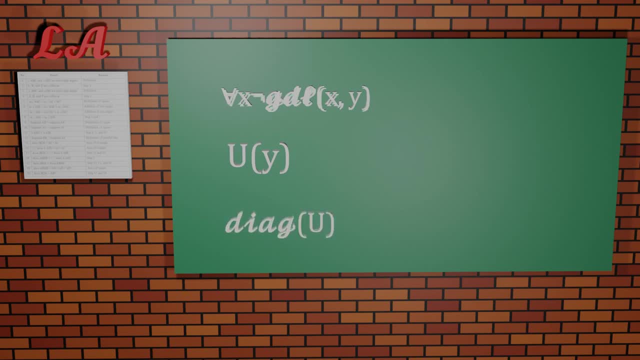 And now diagonalize U, Unpacking this a bit. our formula is equivalent to this, And this is the Gödel sentence for PA, which we've been aiming to construct. we'll abbreviate it G. Consider then what it takes for G to be true. 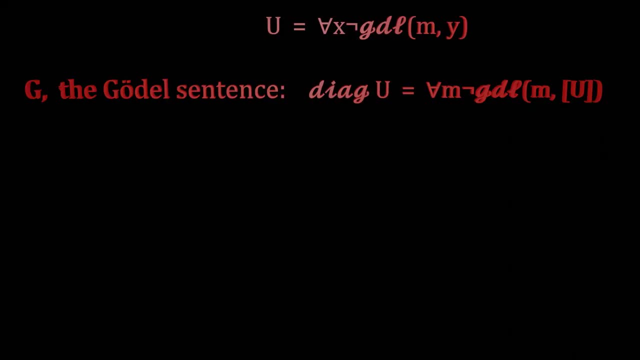 G is true if, and only if, there is no number m such that satisfies this relation. That is to say, given the definition of GLD, G is true if, and only if, there is no number m. that is the code number for a proof of the diagonalization of the formula with Gödel, number U. 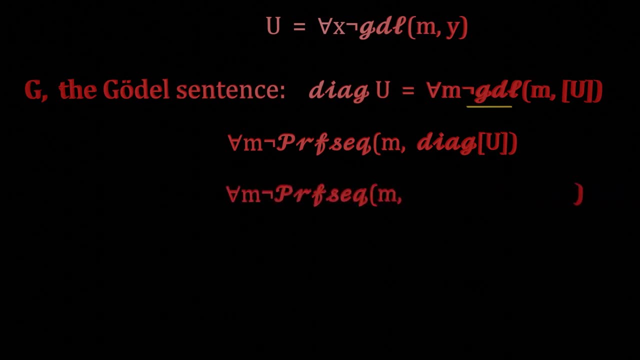 But by construction, the formula with Gödel, number U is the formula U And its diagonalization is G. So G is true if, and only if, there is no number m, such that m is the code number for a proof of G. 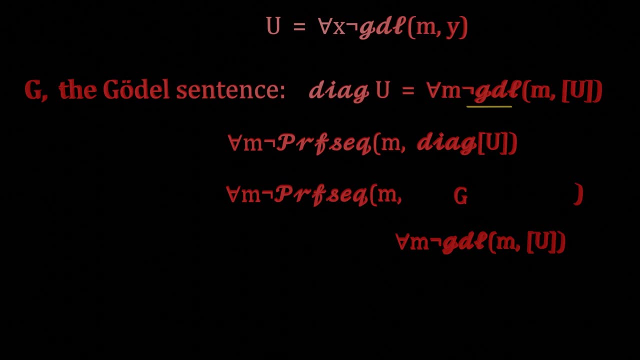 But if G is provable, some number would be the code number of a proof of it. Hence G is true if, and only if, it is unprovable. Wonderful. 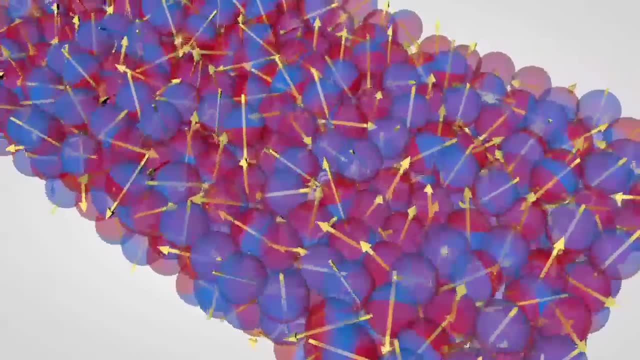 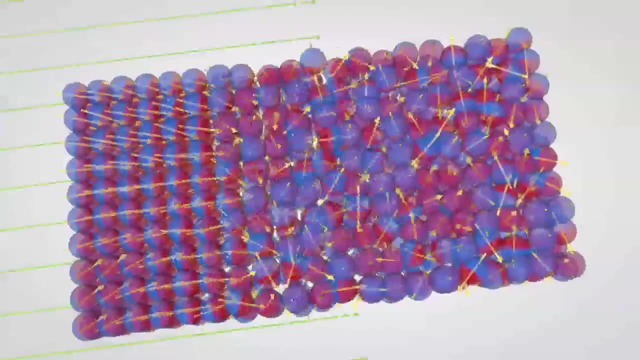 In non-magnetized materials, the magnetic fields of particles are distributed randomly, so they cancel each other out. When the material is magnetized, the atoms clump together into magnetic domains, each with its own magnetic field, Although the domains have a cumulative. 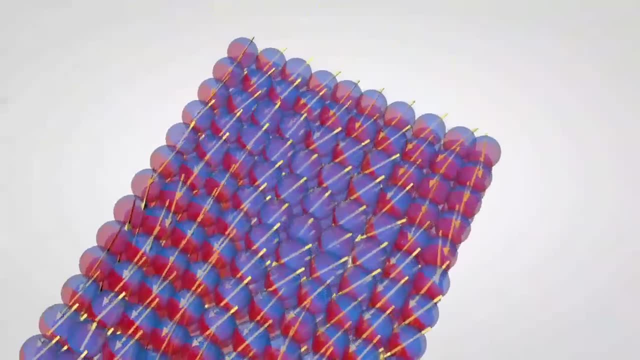 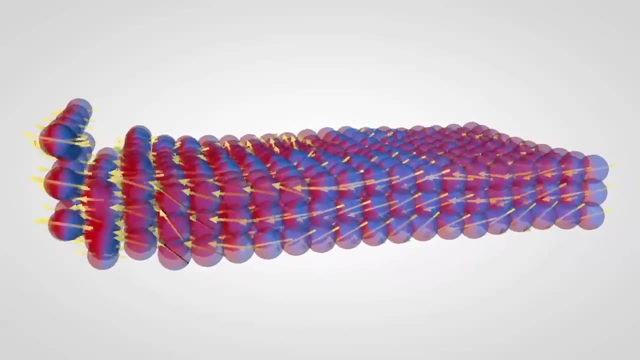 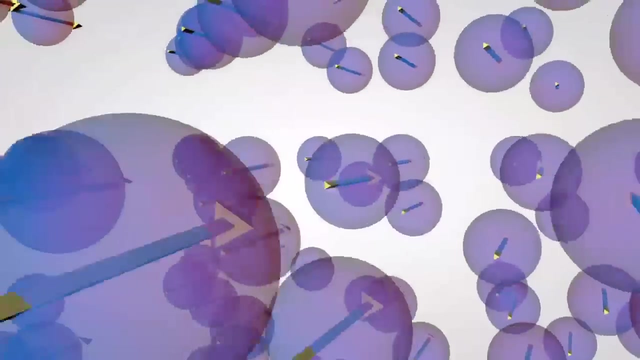 effect of giving the magnet a north and south pole. they are not perfectly aligned, so there's still some cancellation. However, very small particles smaller than a single domain can be arranged so that their atoms work together, an effect called exchange coupling The effect.